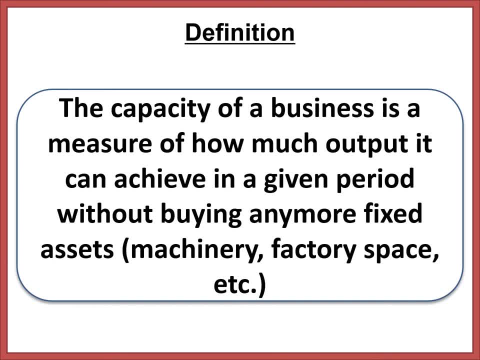 much input it can achieve in a given period without buying any more fixed assets or anything like machinery, factory space etc. So in other words, it's how many like items or how like much like a product can actually be produced in any kind of period of time. 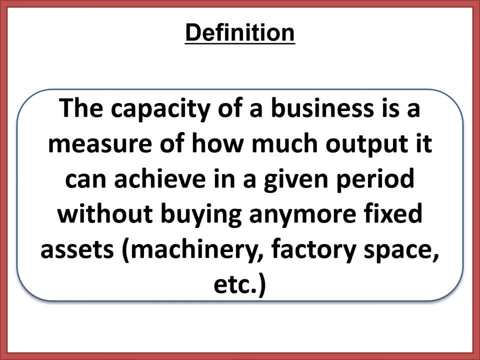 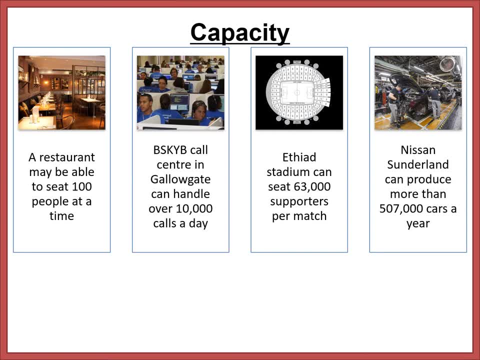 So whether it's monthly, yearly, etc. etc. So if we're thinking about it, so if we're really looking at it, then you'd be looking at like things like capacity for a restaurant that may be able to see 100 people at a time. 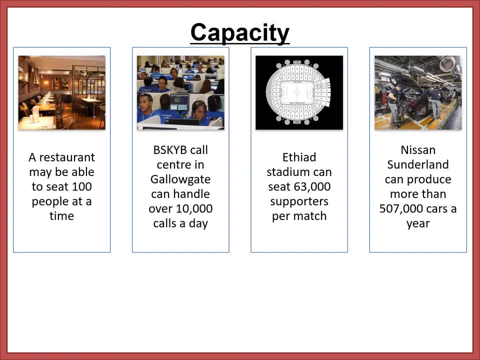 So they can only see 100 people. they won't be able to go any further than that. If you look at BSkyB call center in Gallagate, then they can handle over 10,000 calls per day. So if I'm in the Etihad Stadium can see 63,000 supporters per match, no more, but usually 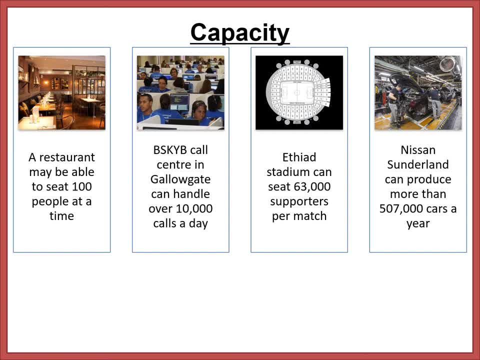 it's less. And then the Nissan Sunderland can produce more than 507,000 cars per year. So that's what we're talking about when talking about capacity: It's how much of a particular unit of like that your company actually produces, how much. 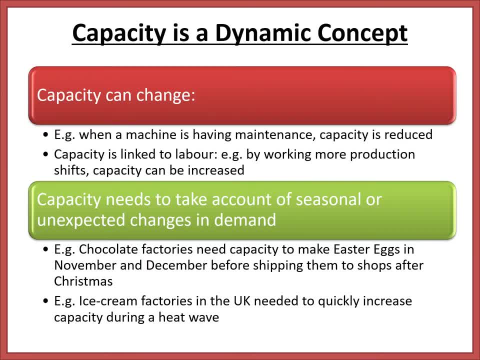 it can actually produce over that time, Okay, Okay. So capacity is actually quite a dynamic concept, so it can change. So if you've got things like say you've got machinery that's gone down, or you have tables out of commission or you have like say with like a football stadium, then maybe you've 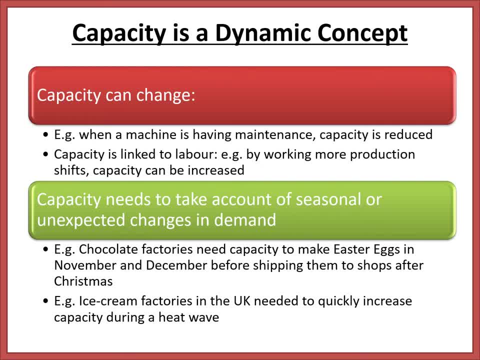 shut down one particular area, then that's going to change your capacity like potential, And capacity is very much linked to labor as well. So by working more, So if you get like more shifts going or you hire more people, then you can actually increase. 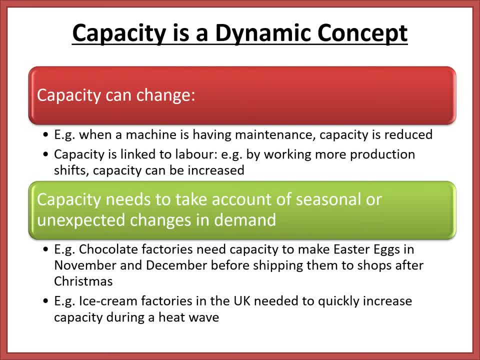 your capacity So it could drop easily when you have anything like maintenance or it can like go up if you start producing more or utilizing the machines properly. So it needs to take account of seasonal or unexpected changes in demand as well. So I mean, like things like chocolate factories need to need capacity to make Easter eggs. 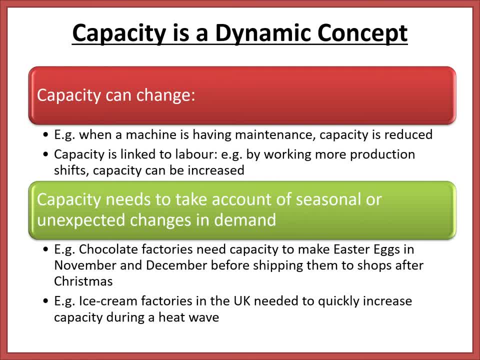 in November and December, before shipping them to shops after Christmas- Okay, Before the actual Easter. Then you've got ice cream factories. So in the UK they need to quickly increase capacity during heat waves and then allow it to reduce down again, And it's kind of like looking at how they actually would achieve these like scenarios. 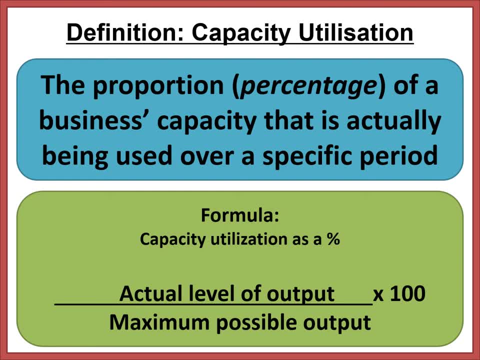 Now capacity utilization. So it's the proportion, It's a percentage of the business's capacity that is actually being used over the specific period. So whenever we look at capacity utilization, Then it should be like expressed as a percentage. Now the formula for it is actual level of output divided by the maximum possible output. 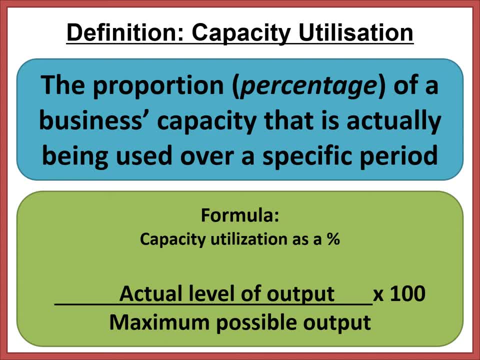 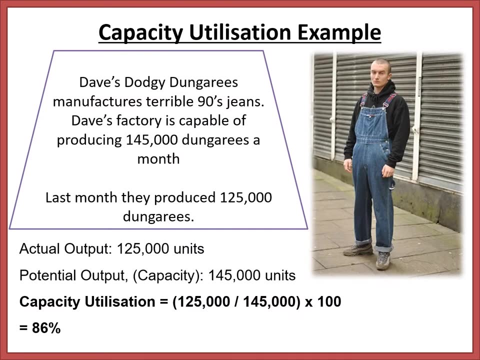 times 100. So you are finding the percentage that a business is actually working at that time by small, usually small. So actual level of output divided by the maximum level times 100. So you can see, here's an example. So we've got dodgy Dave's dungarees. 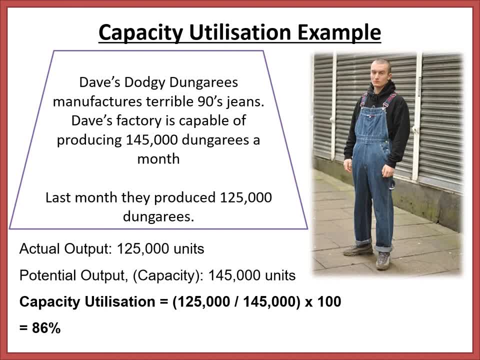 So they manufacture 90s jeans. So you can see there there is a lovely character wearing a pair of dungarees. So Dave's factory is capable of producing 145,000 dungarees a month, But last month they produced 125,000 dungarees. 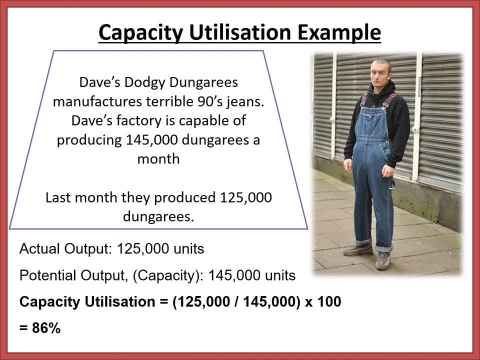 So again, if we go back to the capacity utilization formula, then you've got: the capacity utilization is The Actual output divided by the potential output times 100.. Here we've got 125,000 divided by 145,000 times 100 equals 86%. 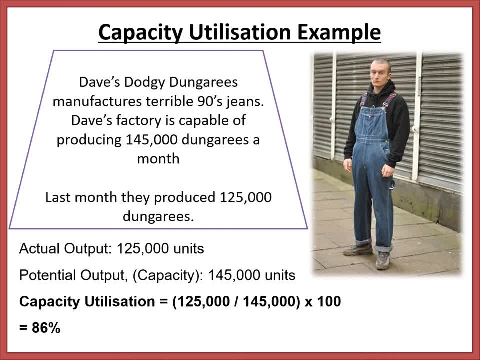 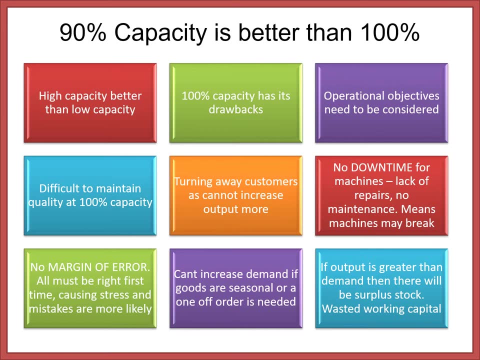 I would usually round this up to: to like up or down to the nearest percent, like actually have it working that way. If you are going to like put decimals in, then just do it to two places maximum. Now, Some companies would seem to think that actually working at a hundred percent capacity is the. 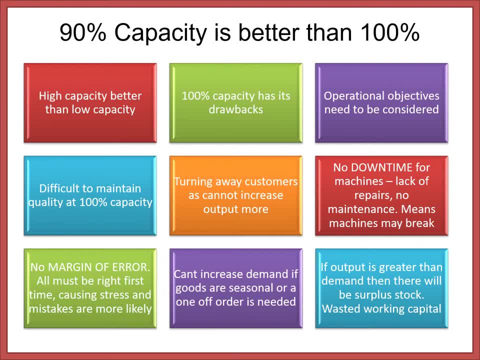 best solution. So obviously you don't want to have any people who are not pulling their weight. You don't want to have any machinery that's not working. You don't want to like be not using all the resources available to actually produce everything that you can. 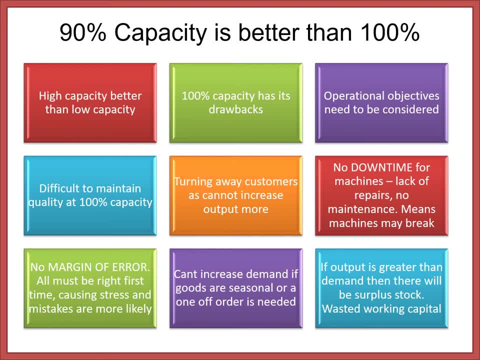 But the truth is that actually, while you do want it to remain high, actually working at a hundred percent has its own problems. So I mean, like, working at, say, around 90 to 95% actually works a lot better, simply because It's very difficult to maintain quality at a hundred percent. 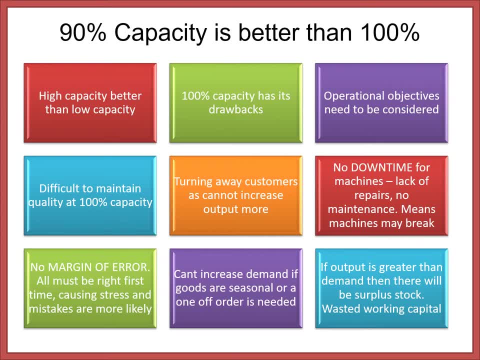 If you are actually trying to push your machines or push your people, it can cause a lot of stress and you end up with like actually people maybe not doing the job that they can do because they're trying to meet targets. But if you had it at 90%, then actually there's a little bit of room there and people might. 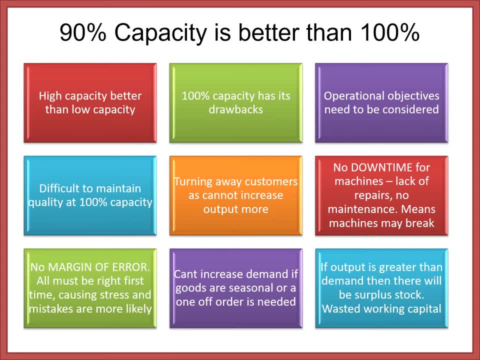 be stressed like might not be stressing, they'll make less mistakes. It also means that you wouldn't be turning away customers. So if you were, say, a restaurant, Then if you are not big enough or you haven't got your tables laid out in the right way, 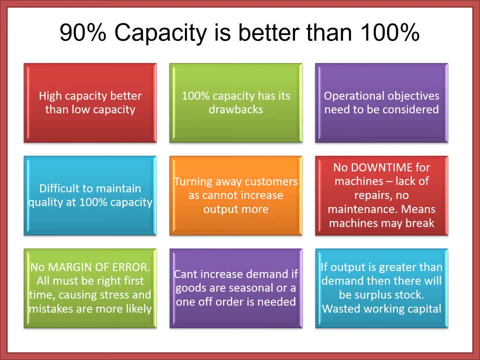 so that you've got enough tables available. then people would turn up And if you're at a hundred percent capacity, you've got a full restaurant. turn people away. They may not come back, And that works for a big shipment orders as well. 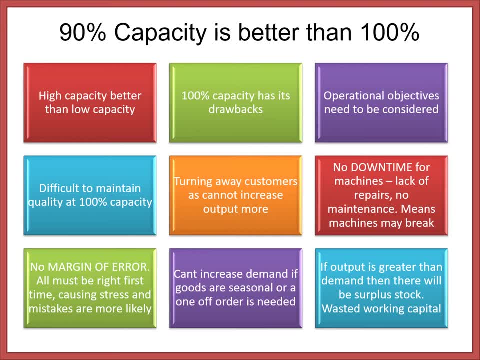 If they, if you've got, say, a small company, and you put right, well, we can produce 150 products a day, and someone comes along and goes right, well, we need a thousand orders for tomorrow, Then you're not going to be able to meet that actual requirement. 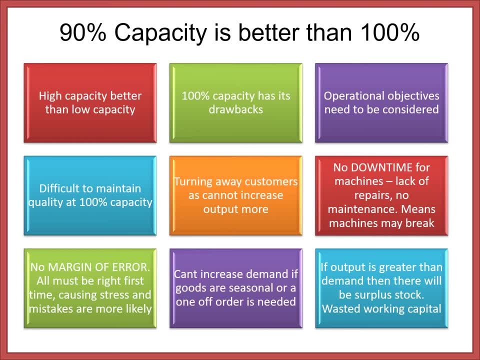 And that could be an issue. Would the people come back to you? Probably not. They'll go to one of your competitors who can meet that need Now. it would also mean that there is no downtime for the machines, So there could be a real serious issue with regards to maintenance. 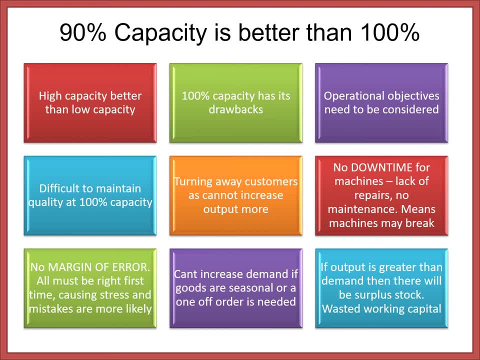 There could be a lack of repairs, And then, if a machine does break, what will happen is everything else will still carry on running and you'll end up with a big backlog waiting for that machine to be fixed before it can all be processed through. 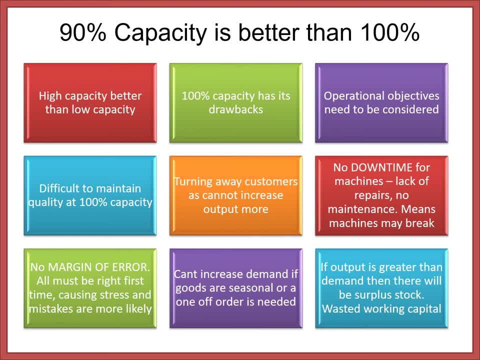 It actually could take a lot longer and the machines could break down a lot more often as well. Also, there's no margin of error. So everything needs to be right first time, because if you've got to redo an order, then you haven't got that kind of buffer zone of right. okay, well, we need to redo something. 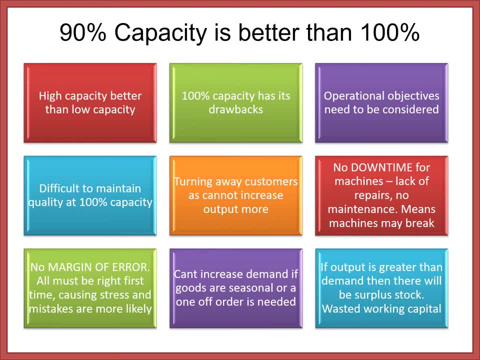 Then it means that we can just sort of put it back into the system and get it done again. It could actually be sent back. You could end up having to like give the refunds on the product and still give the product out as well, And it just causes stress. 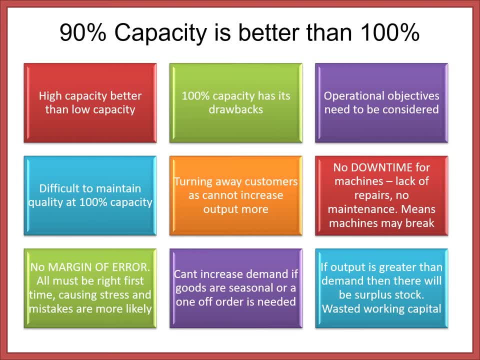 And again, that's where Mm Mistakes can come into it. Also, you can't increase demand if the goods are seasonal or it's a one-off order. So if you are again, if you look at Cadbury's, if they were working to a hundred percent. 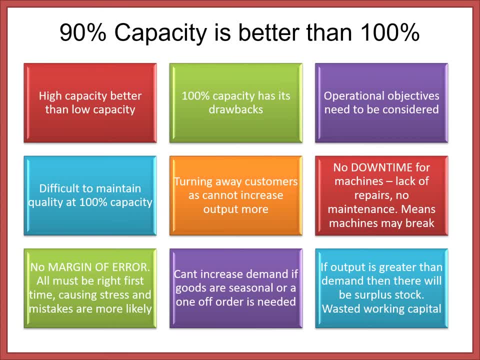 capacity all the time all year, then what would happen when they've got to get ready with Easter eggs for Easter? then they wouldn't be able to sort of move people around. They wouldn't be able to like sort of pull out some of the machinery and really start. 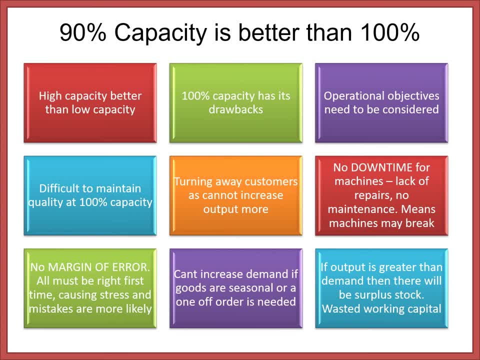 to up the amount of production that's required, because they would have actually been working at the full rate that they can work at all year anyway. And then if output is greater than demand, then there will be surplus stock. So if you're actually working at a hundred percent but demand is only at about 80%, 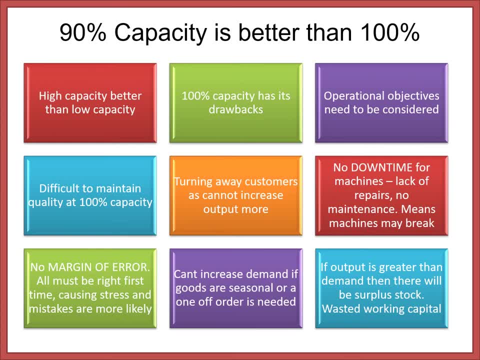 then you're going to end up building up and building up all the surplus stock. People may not buy it, buy it, And then you've got just wasted working capital. That is money that is just sat there not doing anything, not making any kind of profit. 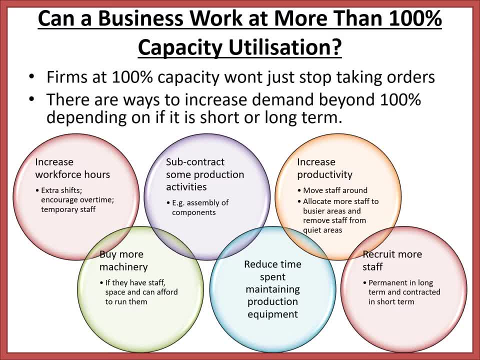 for you. Okay, Okay, Okay. So Well, working out like less than a hundred percent is perfectly acceptable. There are going to be occasions where you may need to actually work out more than 100%. Now I hear you there going like: Dave, you can't work more than a hundred percent a. 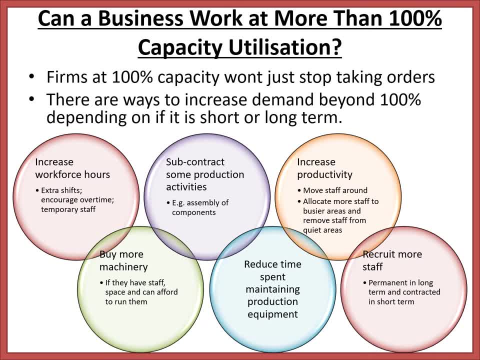 hundred percent is the maximum. Well, there are certain things that you can do. It's if you were working at a hundred percent capacity and someone brought in an extra order for you. you're not just going to turn it away because again they could go to arrival. 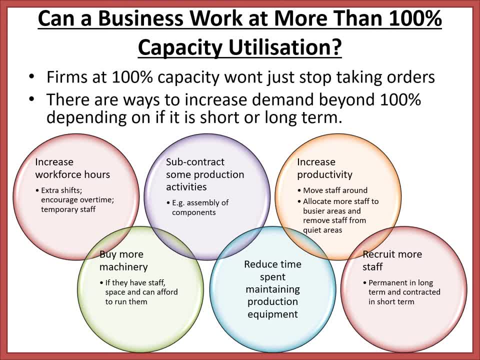 So well, what can i actually do so you could do things like? you could increase workforce hours so you could get extra shifts going. you could encourage people to work overtime. you could hire in temporary staff. you could subcontract some of the production activities so you could actually send. 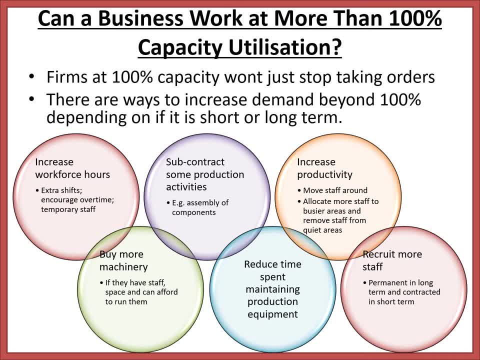 it to another company to fulfill your order now. they would obviously charge you and that would cost you money, but if the extra order is worth it, then that is perfectly reasonable to do. you could increase your productivity. so move staff around. allocate more staff to busy areas and remove them from quieter areas. try and make sure that you've got enough staff that are 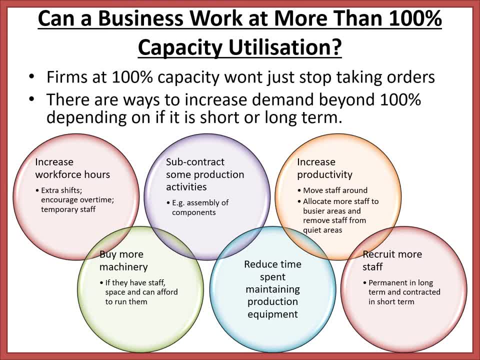 multi-talented or like have multiple skills that they can utilize in other areas, you could buy more machinery. so if you've got the staff and you've got the space and you can afford to run them, then yeah, get another machine in, because then you would actually increase your overall capacity. 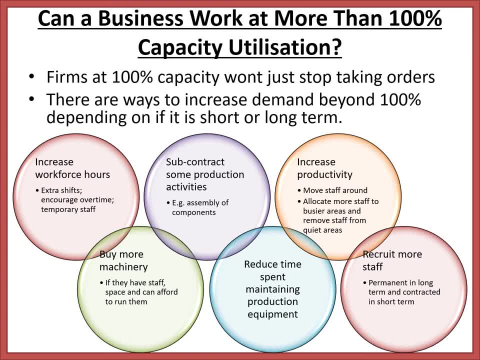 and you could actually be working more- and it's all part of the sort of deal with regards to businesses wanting to grow- uh, you could reduce uh time spent on maintaining the production equipment. so, in other words, you could actually like just sort of make sure that products are working already and sorry, machinery is working already, and then, you know, reduce it. 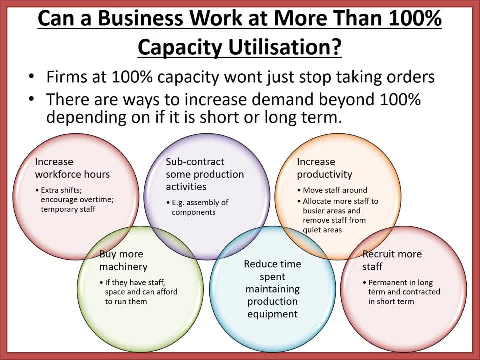 down. now that would come with the risk of, if the machine does break because you're not spending as much time as you need on it, well then what could happen? it could break down, someone could get injured, uh, or you might break down and you wouldn't even be able to fill any of the 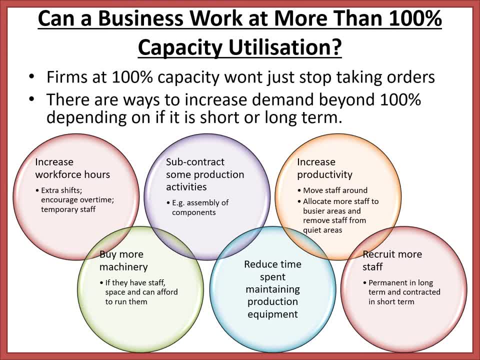 those orders, which again is lost profit. and then finally, it is recruit more staff, so permanent in long term and then just contracted in the short term. so if you know that you are actually like getting any new machines, then it might be a case of right, well, we'll actually hire in permanent. 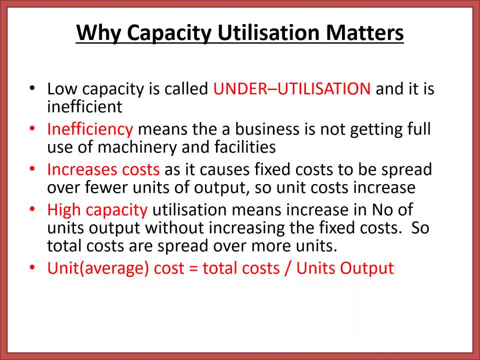 stuff and we'll keep going and keep producing. so why capacity utilization actually matters. so low capacity is under utilization and this is inefficient. now, inefficiency means that the business is not getting the full use of machines and facilities. you are not using everything to its maximum potential right now, if you're at low capacity. 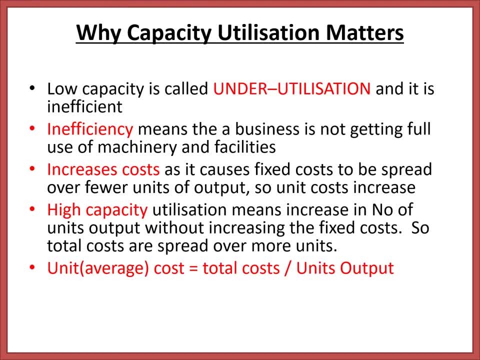 then that means that you might have people just wandering around not really doing much work. you're only using one out of like two machines, when you could have two on, and you've still got orders to fulfill. overall, though, that increases costs, because all of your fixed costs are going to be spread. 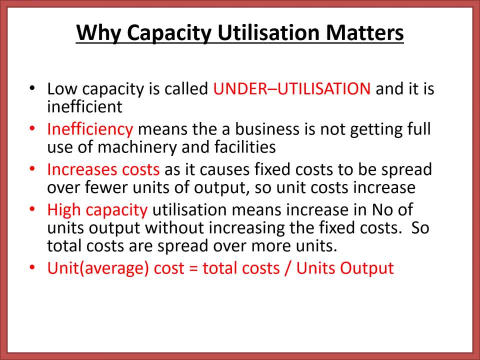 fewer units of output, so no unit costs can increase. so if you think about it, if you are producing uh 100 000 units, and you could be producing 200 000 units of goods, then all of your fixed costs is only going to be spread over the profit that you'd be making. 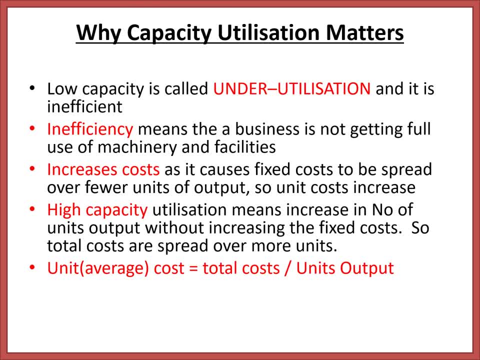 from your uh, the, the revenue of 100 000 units. but if you doubled it then actually they would be, they would go down quite a lot and it means that you could allow yourself a lot more profit in your uh, in your actual goods per unit. high capacity utilization means increase. 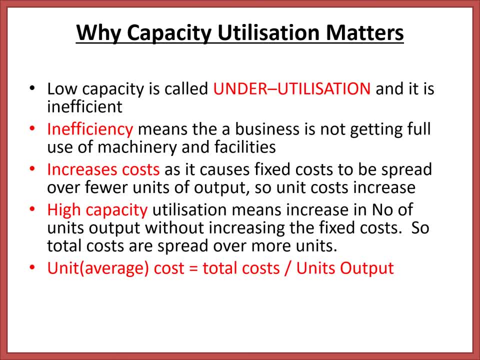 in number of units output without increasing the fixed costs. so total cost is spread over more units and then if we're working out units, so the unit cost is the average. unit cost is the total costs divided by the number of units output. so it's total cost divided by output and that will 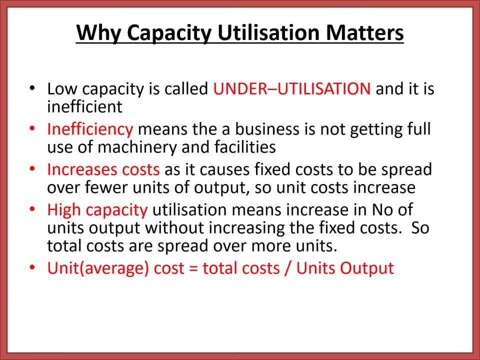 give you your average cost. so if you're working out units, so the unit cost is the average unit cost. so the higher your average cost, the more profit you'll be making. the more like that, the more contribution to your fixed costs would actually be there, which means that you'd be able to develop. 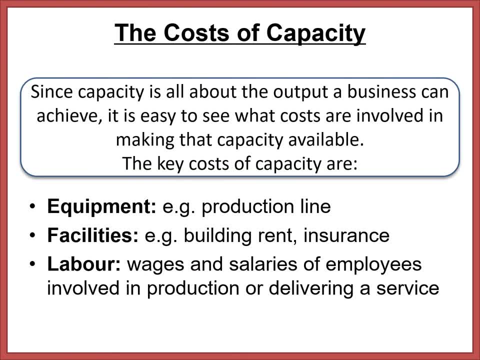 more profit. so cost of capacity. so, since capacity is all about the output of a business, then it's easy to see what the costs are involved, right? so the main ones that we would look at is things like equipment, so your actual production line, machinery equipment, equipment, equipment, equipment equipment. 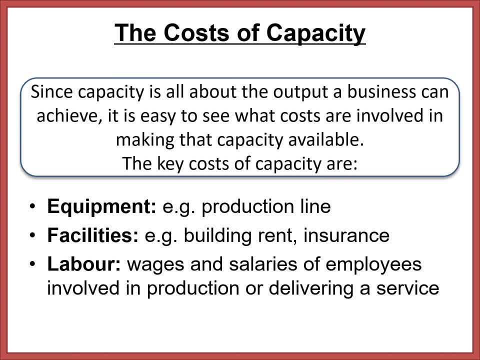 etc. facilities, so building, rent, uh, insurance, like, uh, you know the space that you've actually got, and your labor. so wages and salaries of employees involved in production or delivering a service, those are your main costs. so whenever you talk about cost of capacity, those are the three you need to think about. think about what is being used to produce. 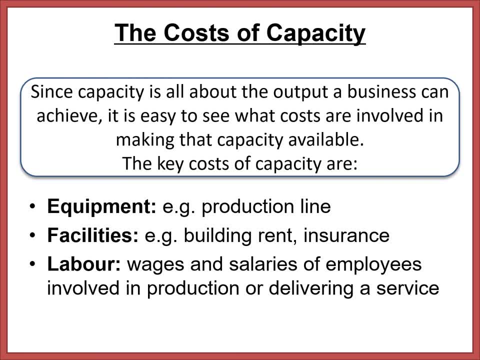 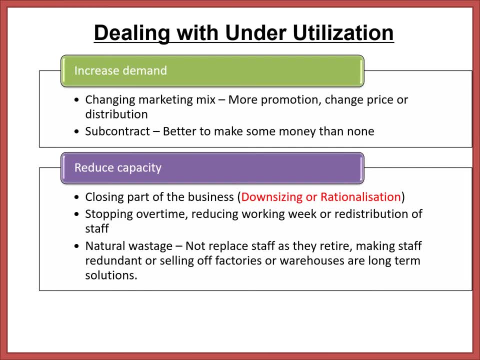 where it's being produced and who is producing it. so how do we deal with underutilization? so what we do is we look at increasing our demand so you can change your marketing mix. put more promotion in, change your prices or your distribution right, get more sales, or you. 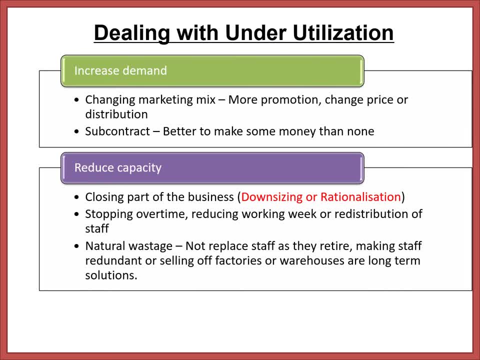 can subcontract. so it's better to make some money than none, right? so if you like need to actually like go out there and get someone else to help you, then do it, or we can reduce capacity. so that would be closing off part of the business. so like downsizing or rationalization. 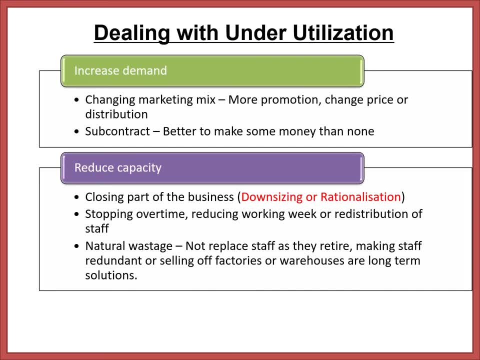 we call this- where basically you could get rid of, um, uh, you could just sort of shut down shops or you can close down like parts of your factory. uh, if you look at uh like some of the energy saving, like ways that uh companies do that to save money as well, then uh, maybe like turning off lights in. 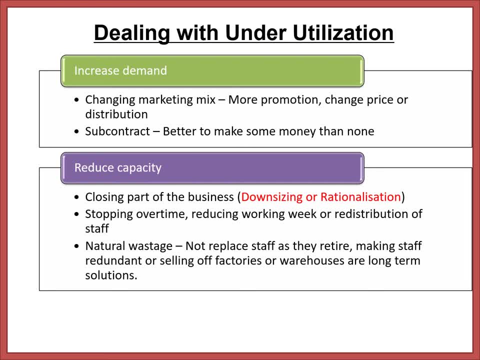 certain areas that are robotic, then we've got stopping overtime, so reducing the working week or risk redistribution of staff. so you know you could actually, you know you could actually, you know you could actually reduce the working week or risk redistribution of staff. so you know you could. 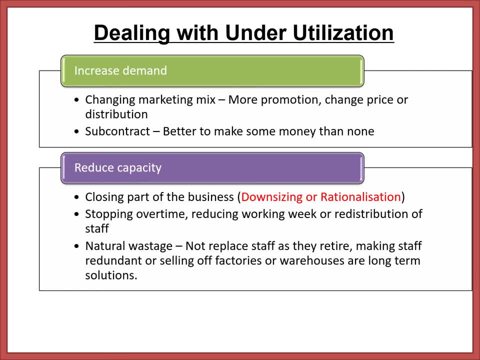 actually not allow people to do overtime, so that overtime is where people work more than their hours. they're allocated usually at an increased amount, so like it could be time and a half or double time, or you could reduce the working weeks instead of people coming in five days. 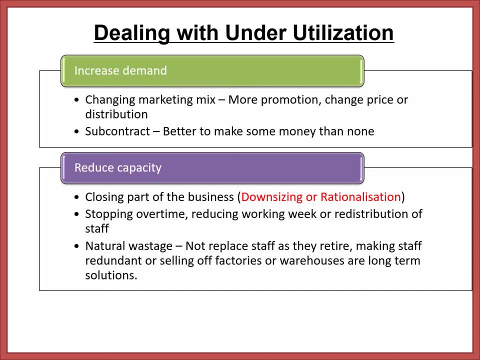 a week, they just come in four. or you could move your staff around the business and actually see: okay, well, if they're not used being needed in a certain area- uh, producing a certain product- could they be moved somewhere else? and then we need to to look at our natural wastage, so as over time people leave, then if you again 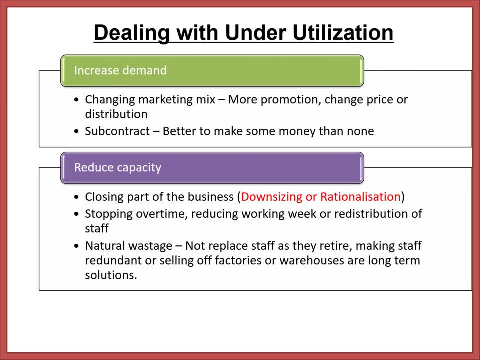 you know that like you're dealing with this underutilization, like you just don't replace those staff, so if they retire, if they are made redundant or you sell off like factories or warhead warehouses over, those are sort of your long-term solutions. so this takes a lot longer to get into play but it just 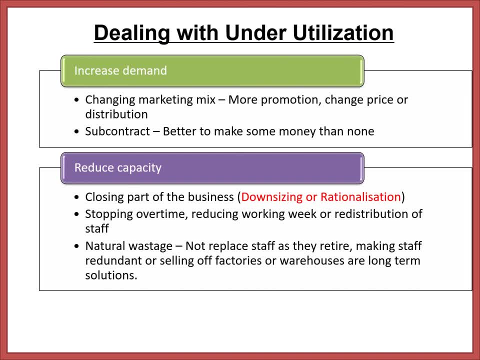 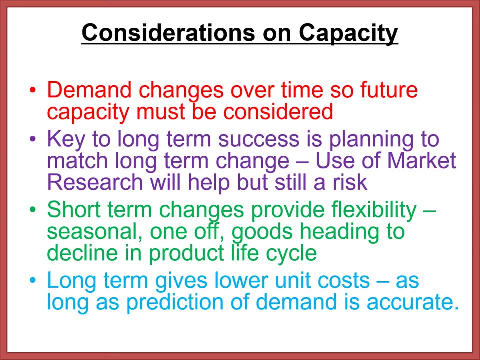 simply means that you allow the company to get smaller in itself, to become more efficient. nothing considerations on capacity, so you've got to make sure that demand changes over time, so future capacity must be considered. if you are seasonal, you need to know when your season is if you are producing an item. 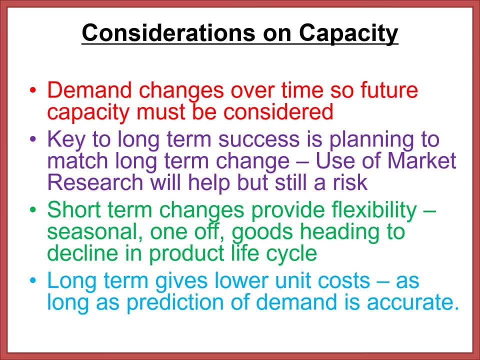 or a product that is going to have a very short life cycle, then you need to know when you need to start producing the next goods right. the key to long terms success is planning to reach to match long-term change. so use of market research will help, but it is still a risk, so you need to actually develop okay. 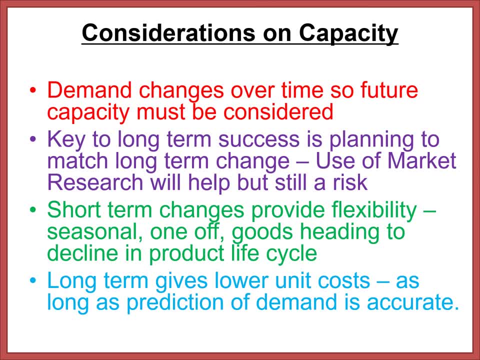 so where are our chain? where is that like market gonna go? is it going to continue on it the way that it is? for example, mobile phones are looking at now developing into foldable phones. are they just going to be a fad or are they going to be the next generation? are you? what is the? what are the companies going to? 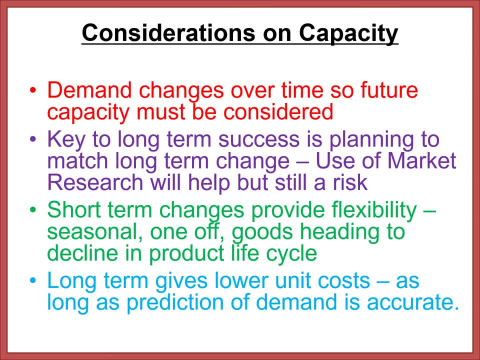 do to actually match that? are they going to all produce one? are they going to get rid of their flagships that they've got at the minute? so short-term changes usually provide flexibility. so things like seasonal one-off, like sales or orders, goods heading to decline in the product life cycle. but in the long term,